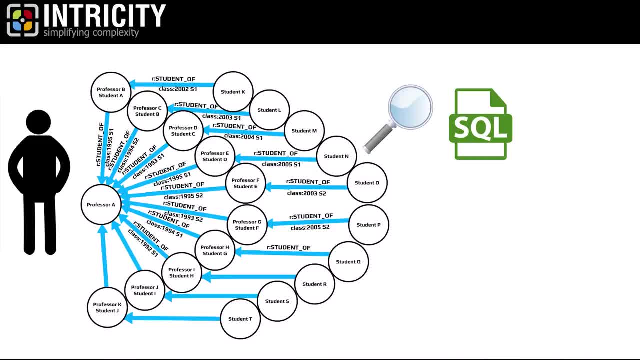 isn't like your typical SQL query. The graph database vendors often have their own query language, so that is something the industry is still working out. And that brings us to some of the drawbacks of graph databases. One fairly obvious drawback is the tendency to get 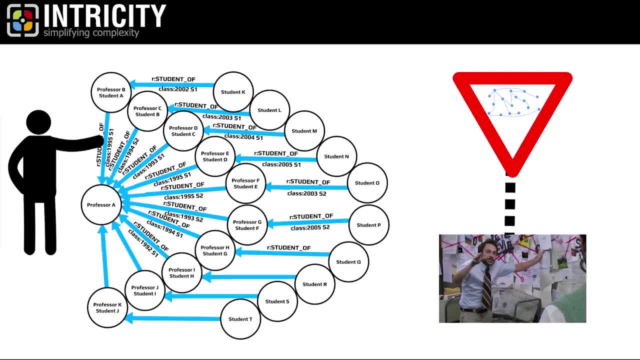 a little conspiratorial, Just as at times the detective board on the movie screen can make somebody look crazy. graph databases can infer connections that really don't actually mean anything. For example, imagine the inference you could make if all the students in our previous 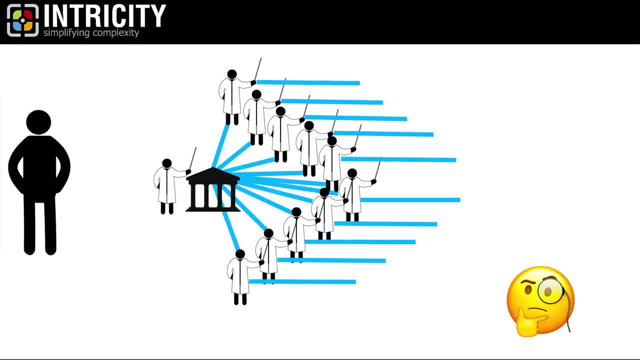 example, ended up dropping out of school. Does that mean that the original professor had some kind of meaningful impact on the university? Or does that mean that the original professor had some kind of meaningful impact on that bad outcome? Well look, anything is possible. 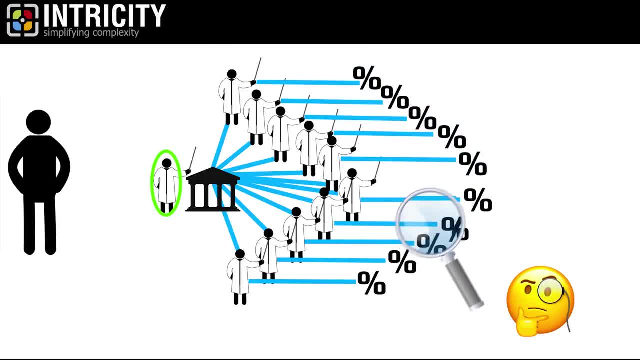 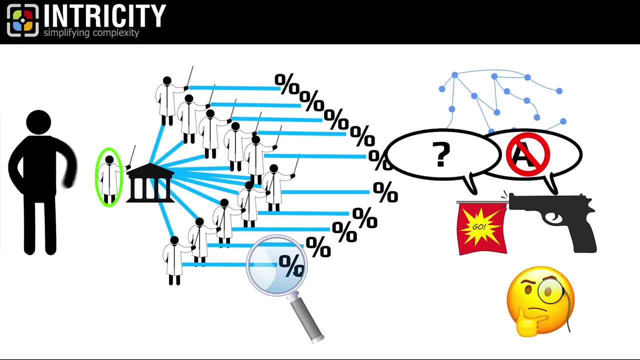 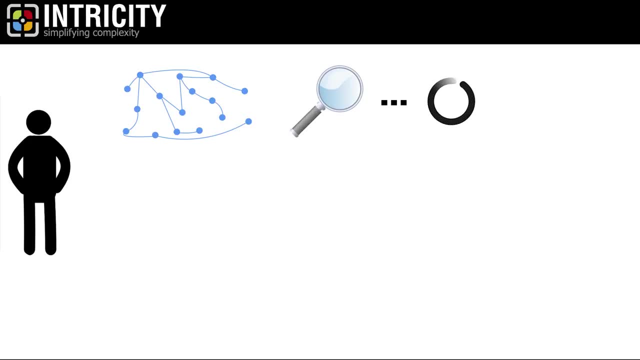 but we have to be a little more skeptical of such conspiratorial patterns. So graph databases are usually a mechanism for starting questions, but not necessarily answering them. Another issue is that it's not uncommon to send a graph database query into an oblivion, often because the query 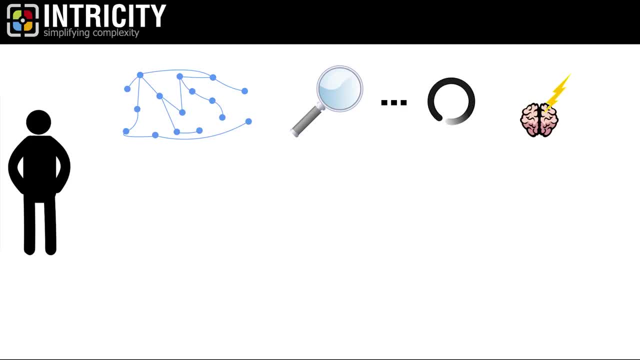 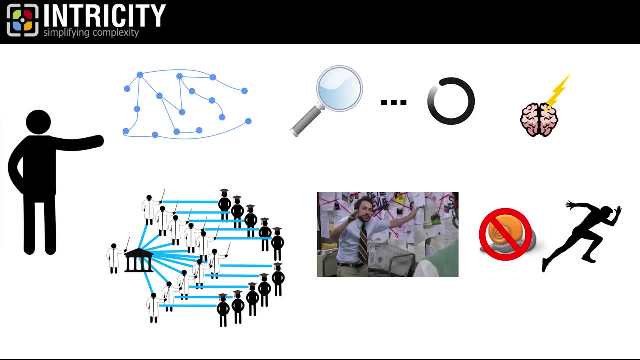 plan can be very difficult to conceptualize. This can lead to incorrect interpretations and slow running queries. That isn't to say that graph databases aren't fast. In fact, for the types of flexibility they offer, they are often the fastest method realistically available. But that speed is tuned to data. 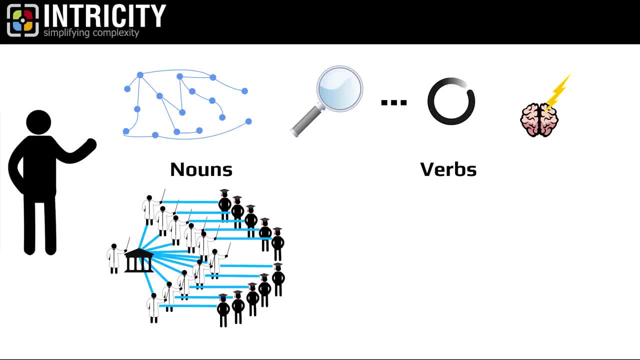 attributes and not transactions, which still remain the realm of relational data warehouses. So what we see is data science communities using graph databases to test inferences. The discovery of these relationships and their relevance to the organization often is what gets bubbled up into the data warehouse. So what we see is that the graph databases are not fast. 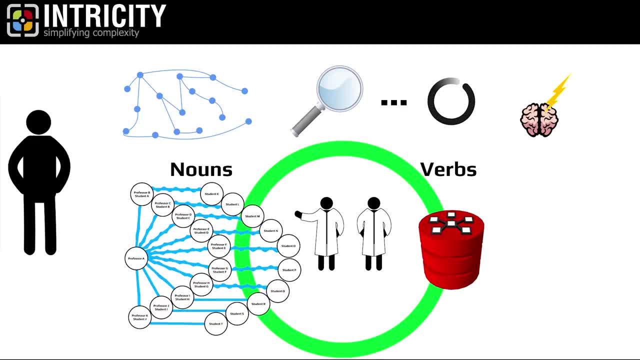 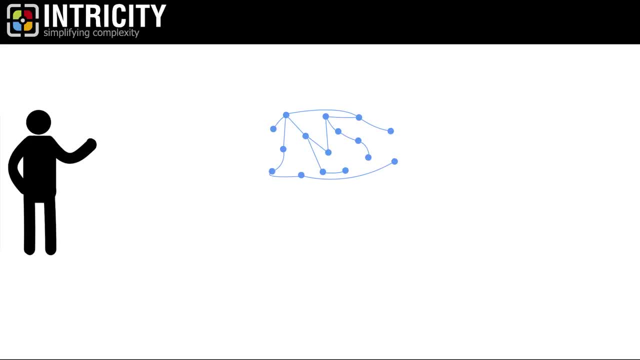 but they are often the fastest method realistically available, Thus closing the loop between the openness of data scientists and orderliness of data integration, like I discussed in one of my earlier videos. So graph databases are a component in a larger landscape of data management tooling. 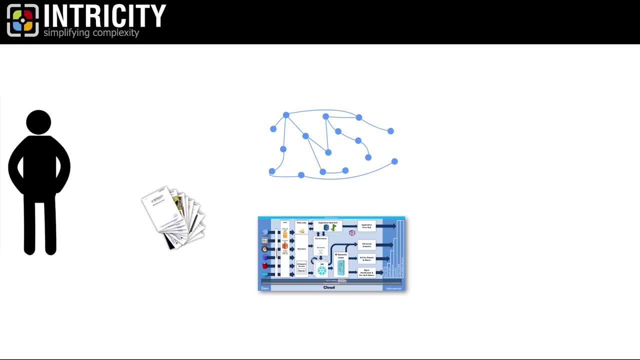 I've written a white paper about graph databases, titled The Data Detective Board, which you can find in the video description. Additionally, if you're considering graph databases in your architecture, you can reach out to Intricity to talk with a specialist.